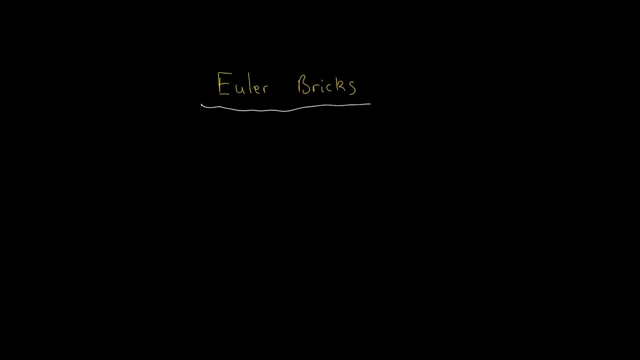 Hello, in this mathematics video we are going to look at the cool concept that is Euler bricks or Euler Euler, however you pronounce it, so I'm just gonna call it Euler bricks, and lower history is named after. it is named after Leonard Leonard. can you guess his surname? it's Leonard bricks, no. 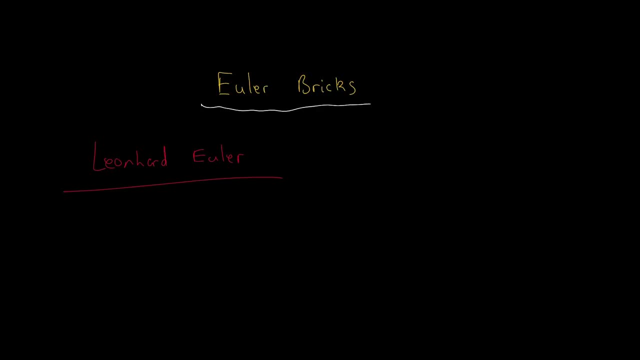 Leonard Euler. so that's basically the history lesson. don't know that I'm joking. there's gonna be a bit more history involved as well. so you might think: what is an Euler brick? and just to confirm, just to confirm, when I talk about bricks, I am talking about essentially this: this shape. 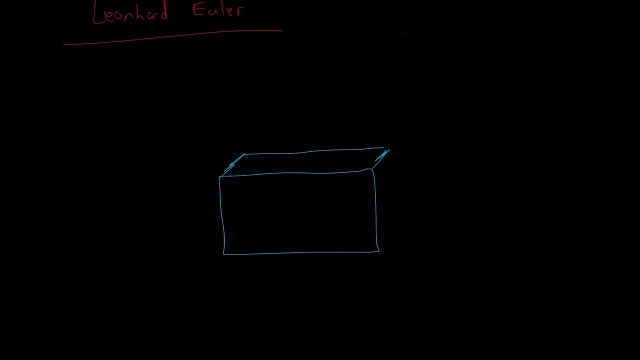 this form factor. this isn't necessarily an Euler brick, but this is a brick, sort of bricks that you would use to make a house, make other buildings with this sort of essentially cuboid, as it is known, this. yeah, that was terrible. this cuboid is a brick. again, like I said, this isn't necessarily a Euler brick. I can. 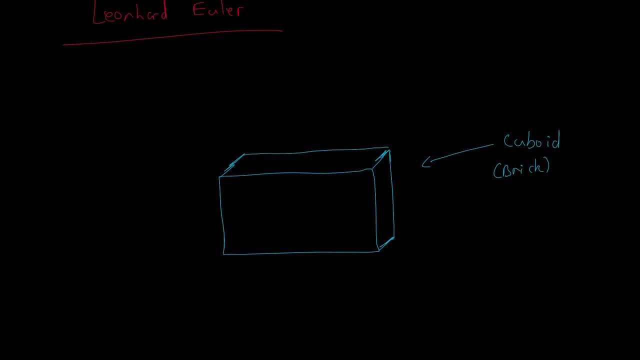 guarantee you, very most likely is not. and a Euler brick is one where all of its sides, all of its sides- i haven't put lines over the other sides- simply because with a cuboid there are only three unique side of three potentially unique side lengths, because there 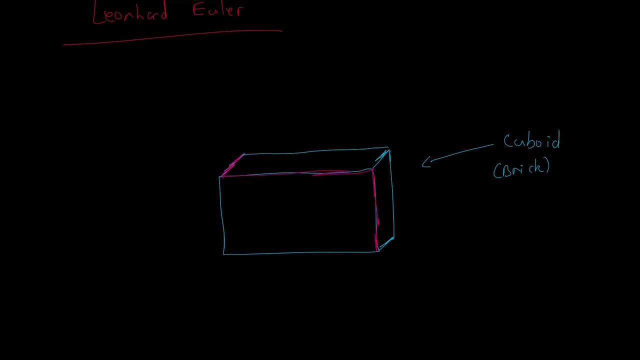 are only three pairs of faces, even though there's a total of six faces. so there are only three potentially unique lengths on a brick and each one of them has to be a whole number. so each, each one of them has to be a whole number. i'm thinking, okay, that is some bargain, easy draw. 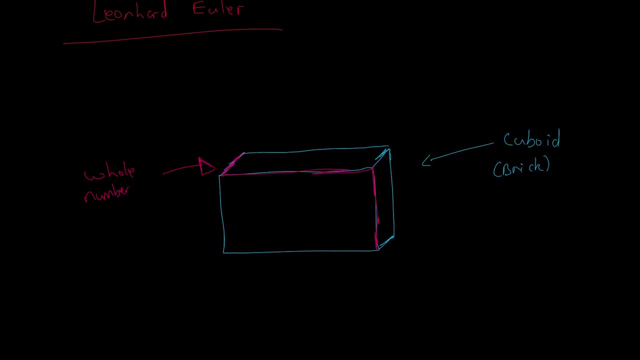 a brick where each one is a whole number. we can actually just sort of label it now. so let's label that four, label it six, label it seven. so, oh, we don't know, this still isn't an oiler brick. there's still actually one more. one last part. 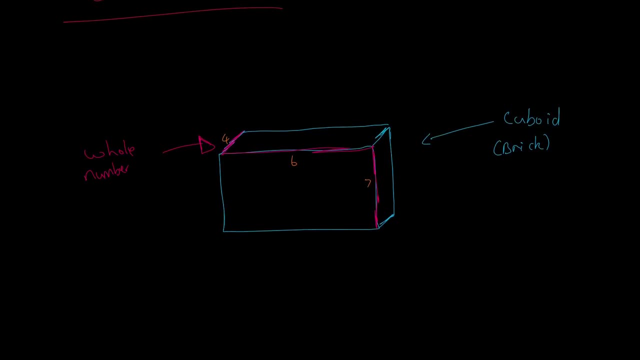 for it to be considered an oiler brick, and it is this the diagonal diagonal of that. no, that was terrible. i want to redo that line. please let me redo it, that's okay. the diagonal of every single face. again, there's only three unique faces, potentially because there's three pairs of faces, hence why i've only drawn three lines. 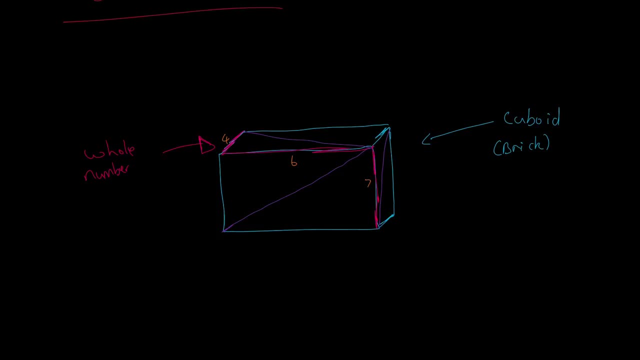 each diagonal also has to be a whole number as well, and you would work this out using the pythagoras theorem. so if we just did a some basic- actually you know what before we do the pythagoras with this? so i'm going to show you some simple square pythagoras. so, to have a look, let's have a. 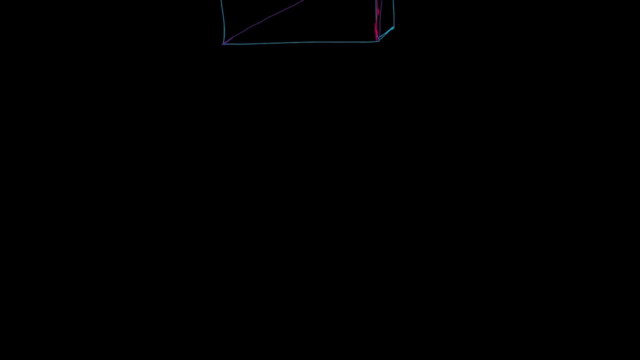 look, could our perfect- i mean our oiler brick- be an oiler brick? so let's have a look. could our perfect- i mean our oiler brick, could our perfect, i mean our oiler brick- have a face? that was a square. so if we have a square and we have one by one, what is its? 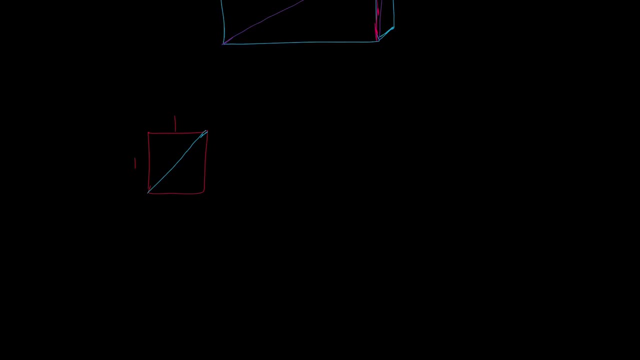 length and we can work that out. i'm going to calculate in my hand: one squared plus one squared is equal to two and the square root of two is not a whole number, it is one. and the square root of two is not a whole number, it is one. 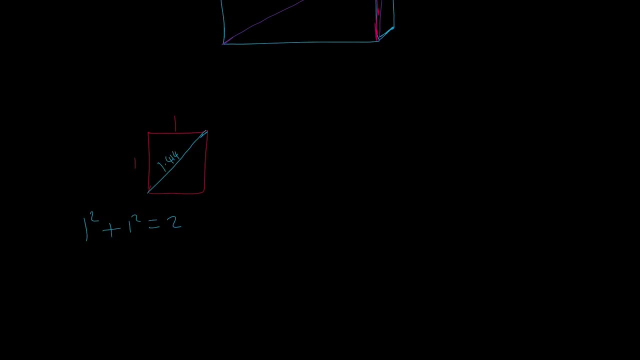 point four: one four, and there's a bunch of other digits, but it's not a whole number, so that is not valid. let's move up one. let's just move to a slightly bigger one. this isn't a scale, by the way. two by two. i don't know what happened here, so these are meant to be squares, by the way, even though they're not. 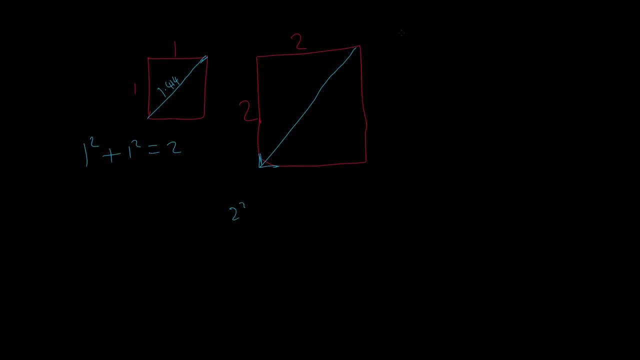 accurately drawn a square. so this is two squared plus two squared, which equals eight. so the square root, the square root of eight, is two point eight, two. i'm just going to do it all to three decimal places, assuming there's three or more. two point eight, two eight. now let's have a look at. 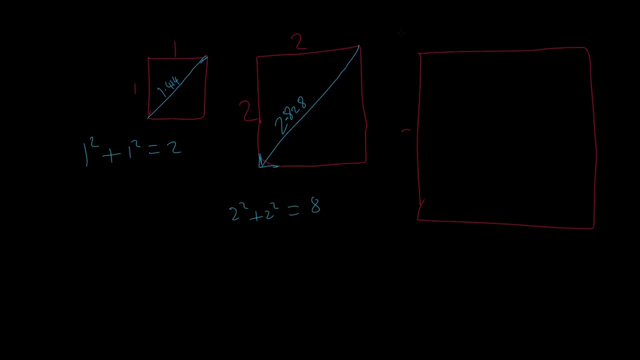 three by three, so three by three, and that's three by three squared plus three squared, which equals eighteen, because this part is nine plus nine, because eighteen, so three squared. so square root of eighteen is: is three times the square root of two, which equals four point two, four, three. again, just round it, three decimal places, so four point two, four, three. 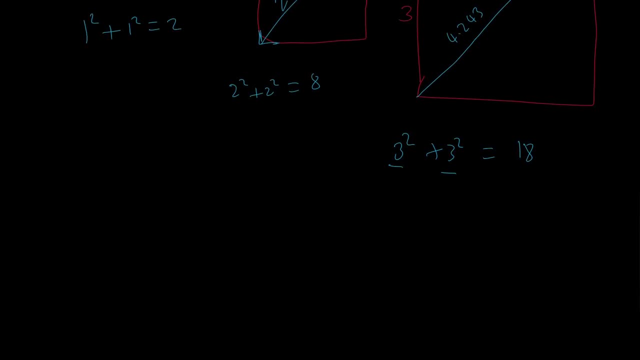 four point two, four, three. i'm just going to do one more, and i think you guessed it, it's just going to be. it's going to be a four by four. four by four and four squared plus four squared is equal to 32, because this part is 16 plus 16 equals 32.. 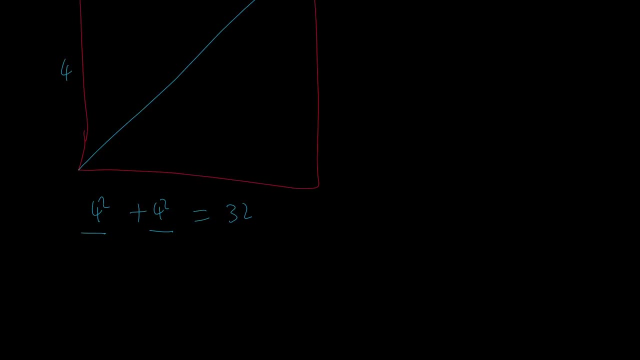 the square root of 32 is four square root two, which can give us a value of five point five point six two, five six seven, again still not valid, and this is just for a square. mathematicians have determined that there is no square that has all of its sides. 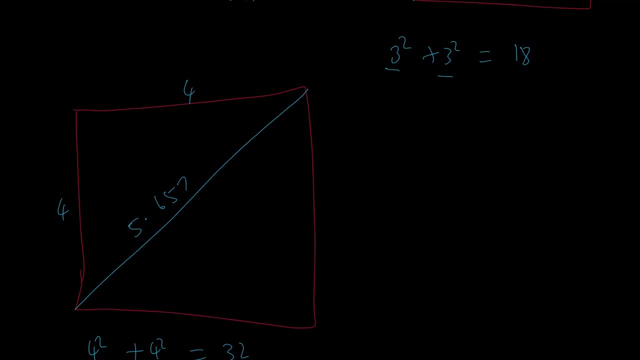 the same. obviously it's all right, besides, also anything square, but its sides there are a whole number and It's diagonals that are a whole number as well. So far there. potentially, may mathematicians may discover one. This is always the way with maths and science. 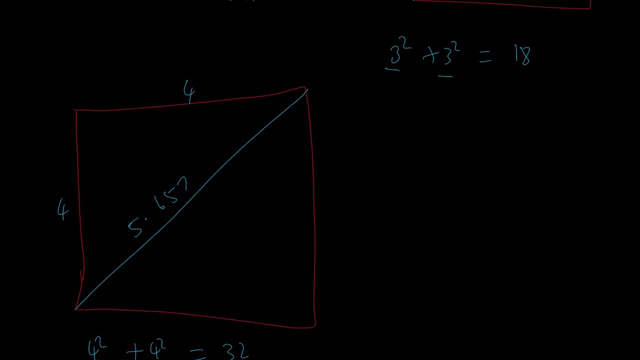 New innovation, whether it's technological innovations or some new way of thinking. Certain things get disproved. certain things get proved, But so far it looks like there is no square that has a diagonal. Well, that is a whole number, So let's get on to rectangles. 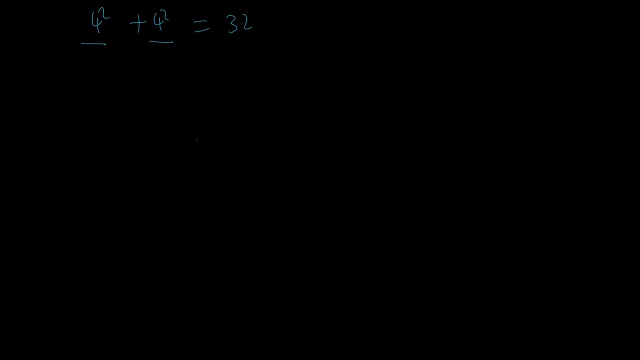 Spoiler alert: there are. So if we do this rectangle not drawn to scale whatsoever. So if we have a side of 3,, 4, this is the most basic example that you are taught when you learn about Pythagoras. 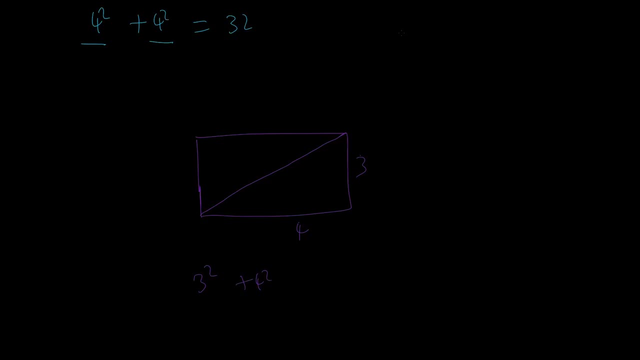 So if we do 3 squared plus 4 squared, this part gives us- I'll actually do it like this- This part we're going to slightly bigger number now equals 9.. This part gives us 16, and then together we get 25. square root of 25 is equal to 5.. 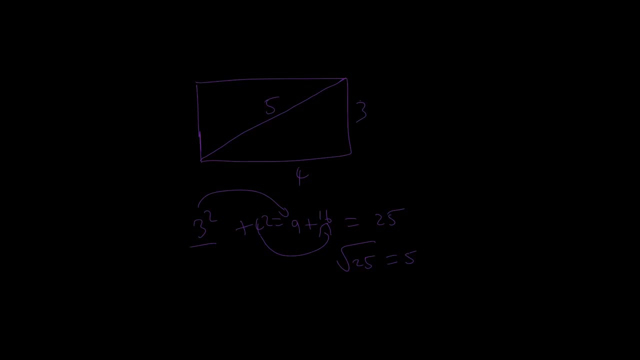 So, yes, this has a diagonal that is a whole number, and its sides are also whole numbers as well. Some other acceptable. Well, some other acceptable rectangles, again not drawn to scale, are 5 by 12 and this results in 13.. 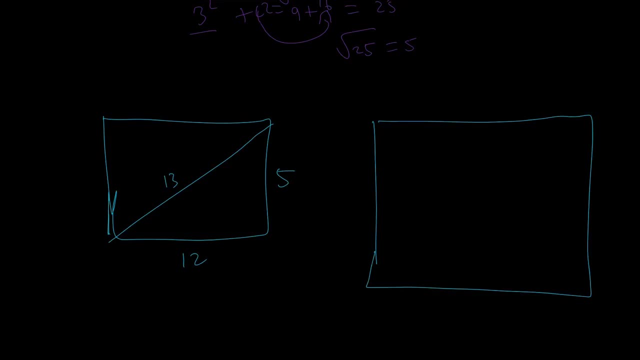 You can do the calculations to confirm, but I think you get the picture of what we're doing, Just basic Pythagoras. That was a terrible line. Much better. Oh, that almost looks straight, especially in the middle part. I'm actually very impressed. 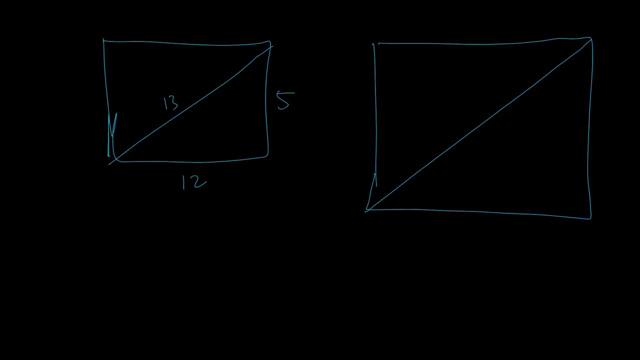 By the line, if nothing else, from this video I got a good line, but this is 25,, 24,, 7, and I'll provide one more, Why not? And this is 17,, 15, and 8,, so 8 by 15 has a diagonal of 17,. so that's all good, but so far we don't have a brick. 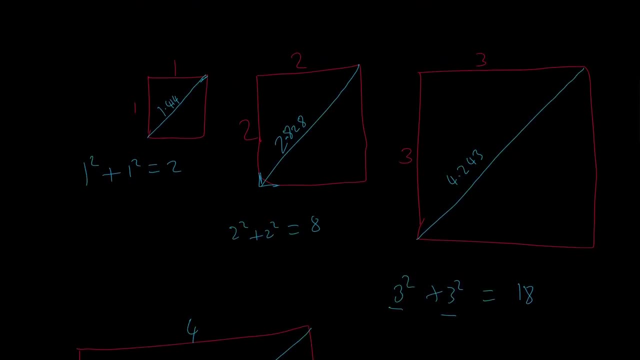 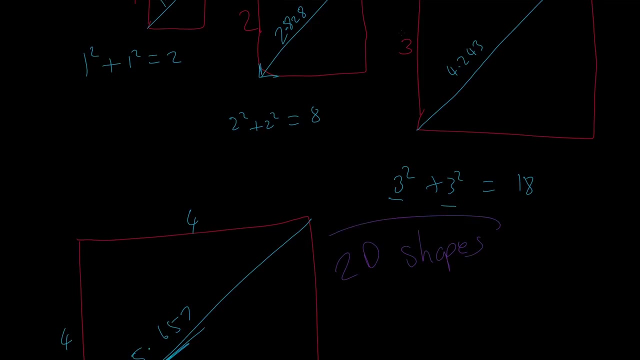 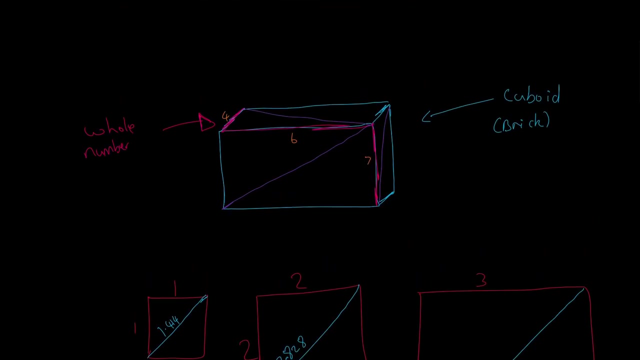 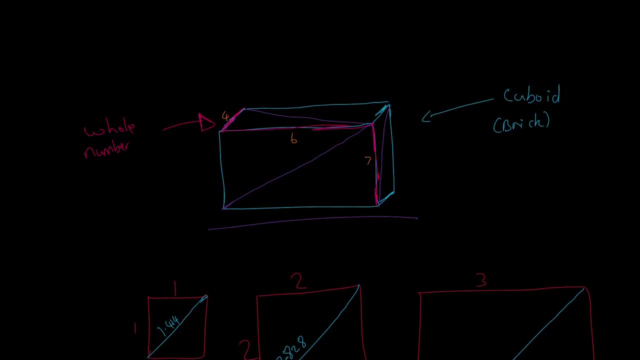 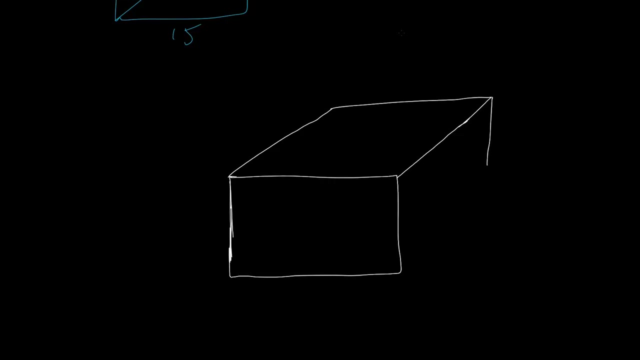 So if we were to put a bunch of these together, we can try and work it out, but already have looked at what the smallest, smallest oiler brick is And the smallest boiler brick is one. I'll draw it out again. I will draw it out again. it is one where 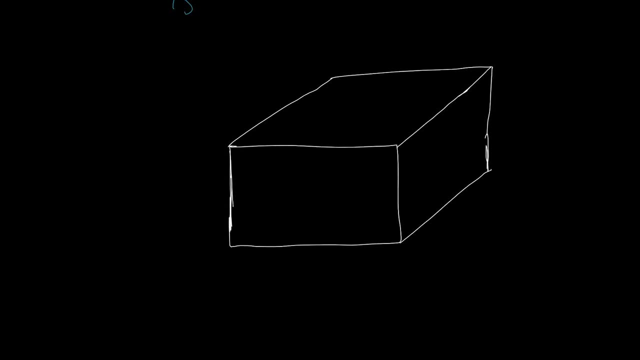 it's height, so it's height, so this value here this side is 44, its width- this over here- is 117, and the length, so I'm going to choose a better color. that's not the best color and its length. 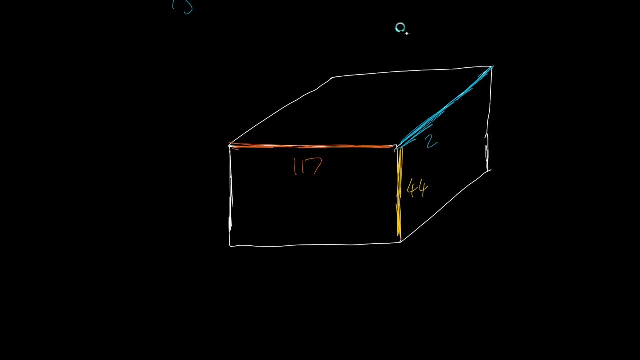 over here is 240. so if you were to try and just well work these out, so let's just, i've already got them worked out so we can have a look. so this one over here. so the side that is 117 by 44 is 100- 125. so this is 125. i'll actually draw it with. 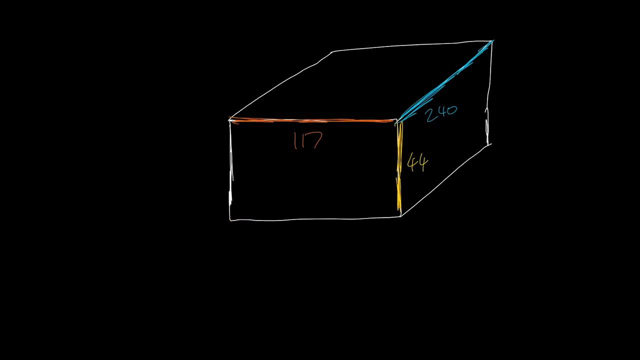 this. i'll actually draw it with a green color, so this will indicate all of the diagonals. this is 125. let's have a look at the other side. there we go. that is 44 by 240. so 44 by 240 is the longest side, or the second longest side, I should say. 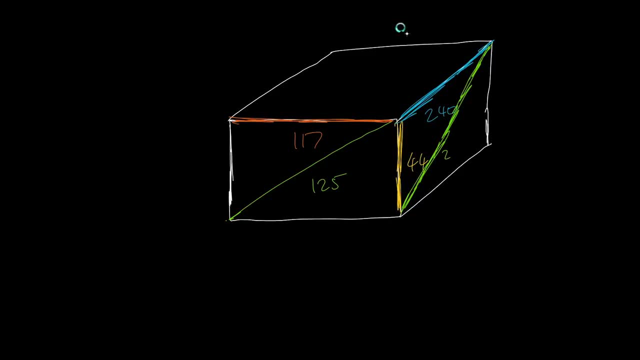 and that produces a diagonal of 244. so 244. so that's the diagonal there. and now the longest diagonal, which is this one over here. now I can draw a better line than that. yeah, that's probably the best I'm gonna be able to do it. the longest diagonal here, which is the diagonal for the side. 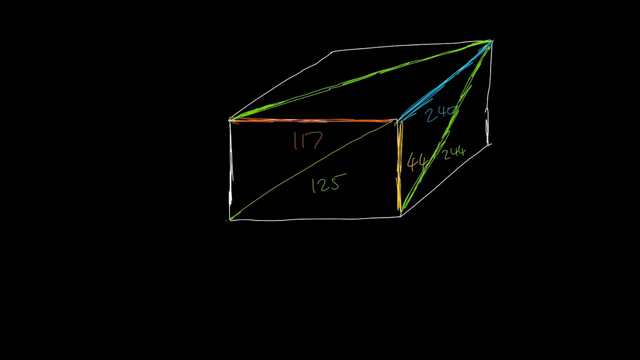 117 by 240 produces a hypotenuse, as it is known in Pythagoras, of 267. so this is the smallest Euler brick. see if you can find a smaller one. compute, I mean, mathematicians have used computers over the years to see if they have. they can find one and they have not. so this is the smallest. 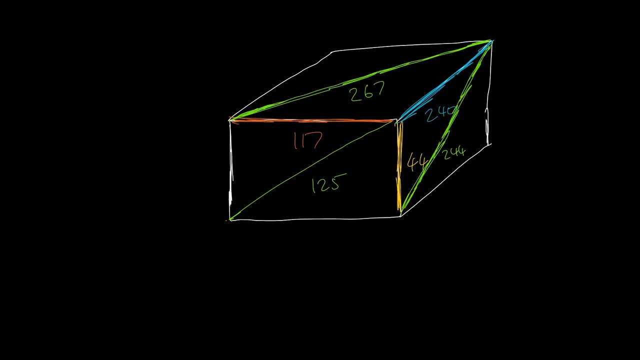 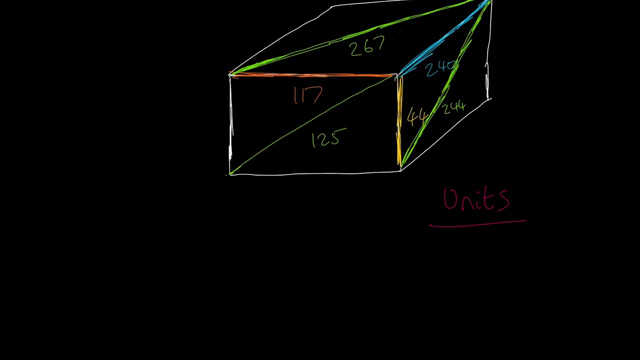 perfect Euler brick also. one thing I wanted to mention- so don't think I have in this video so far- is I'm just using just units for these values. they're not in centimeters, kilometers or anything else. it doesn't actually matter what unit it's in: it could be centimeters, kilometers. 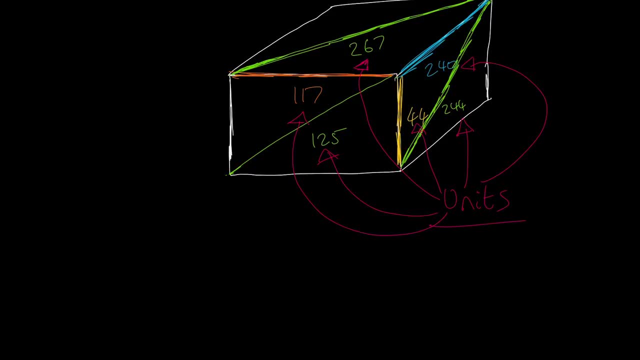 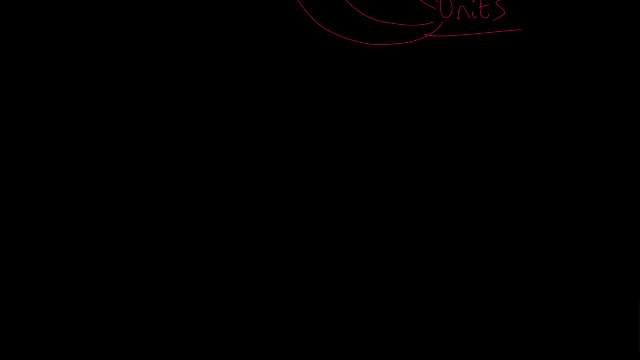 yep, kilometers long and centimeter, but a whole number is still a whole number. that's a Euler brick. there's an even cooler concept, and that is- and this, this mysterious object, is called a perfect Euler brick, and a perfect Euler brick is one where? so let me just draw a brick out. 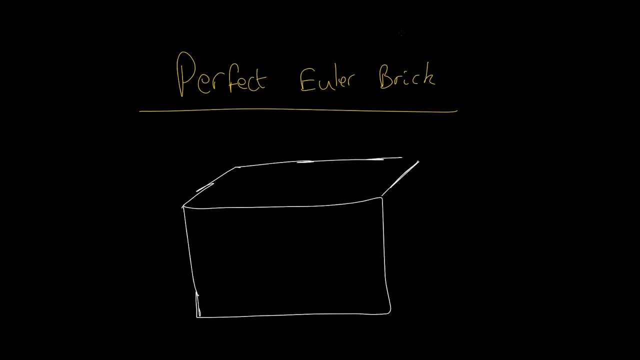 it is one where not only are its sides and whole numbers, not only- let me do a different color for this- and not only are its diagonals of all of the faces, they not only are these. using Pythagoras you can work them out, whole numbers- but 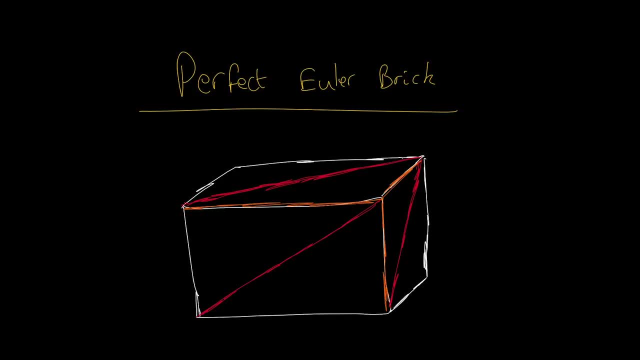 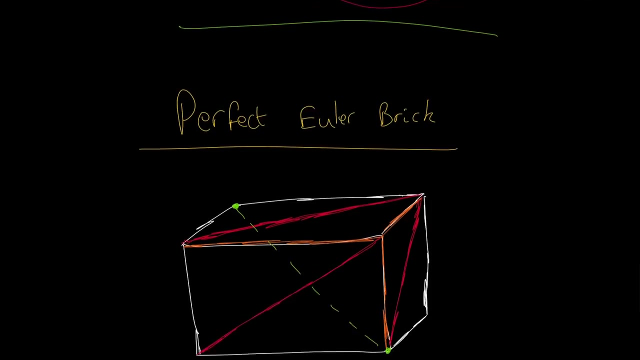 but, but. but. so is the diagonal from one corner to the opposite corner. so this invisible diagonal that would be going through the shape is also a whole number. and, as we or you might be thinking, as I did with this Euler brick, I will now be giving you an example. and no, it won't be, because a perfect Euler brick has never been. 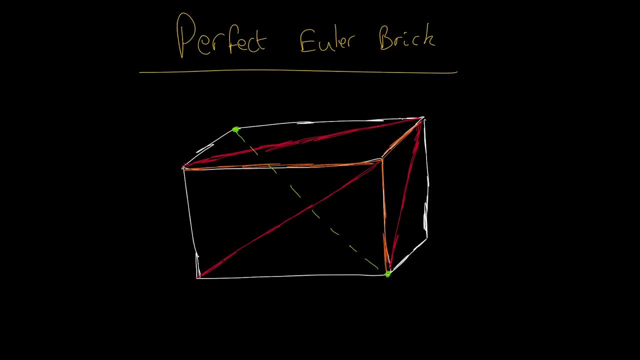 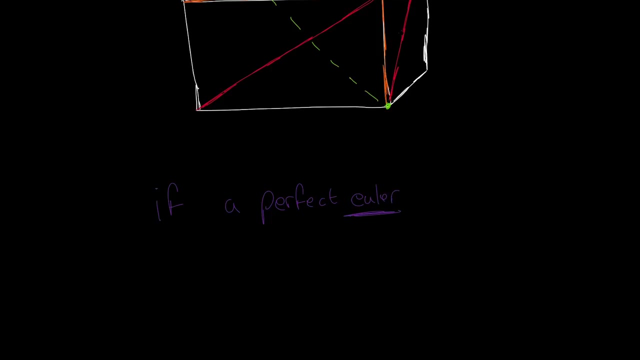 discovered? not at all, even with the power of computers. mathematicians have worked out using computing power, with, with all, like the immense power that we have with computers today. that if and- and this is a big if- if a perfect, a perfect Euler brick exists, exists, then at least one of its sides? 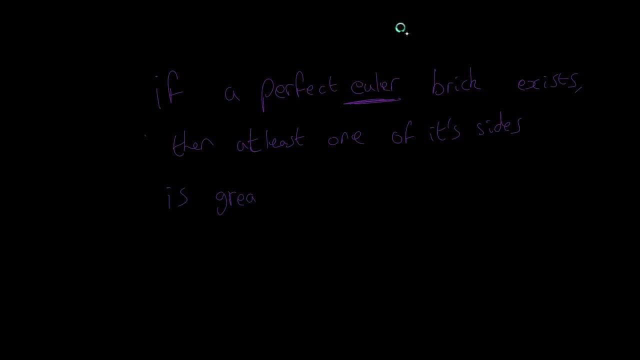 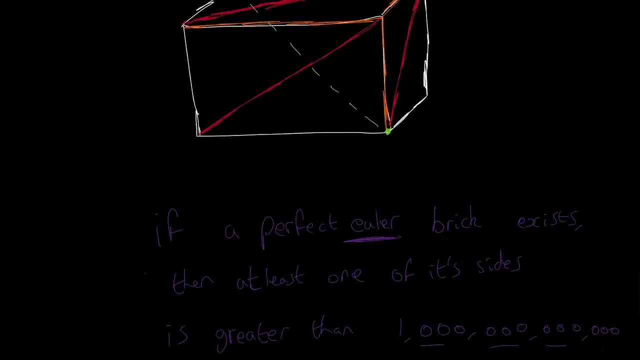 sides is greater. drum roll please. so that was like a terrible drum roll. it is greater than one trillion units, so one of the sides that is. so it is greater than one trillion. so thousand million billion, one trillion units. that's much bigger than the numbers that we've been dealing with here. so 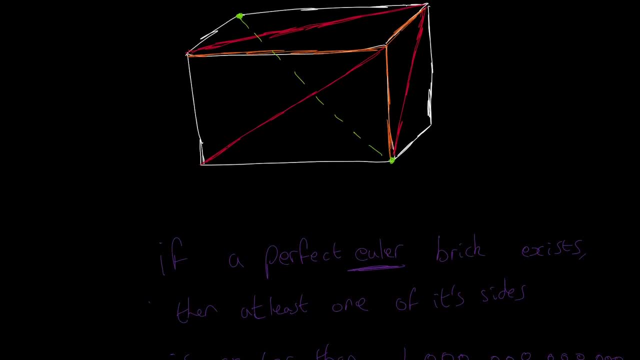 mathematicians so far have not found the perfect Euler brick. if you think you're up to the challenge, I double dare you, I triple dare you. I, Euler, dare you to see if you can find a perfect oiler brick. the maths community, the scientific community, 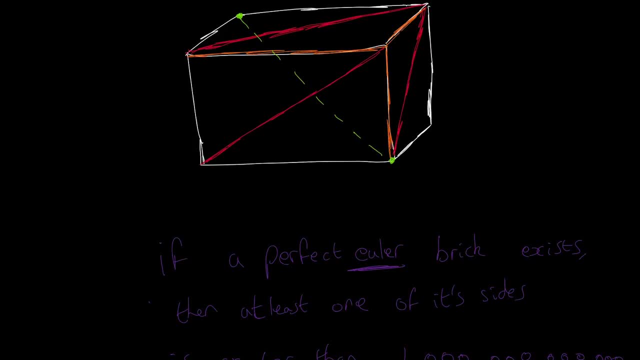 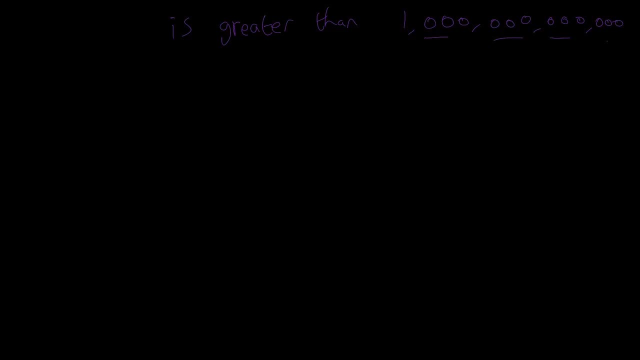 will go crazy. they will hail you as a deity if you can. the closest thing- actually, before I close up, closest thing- to a perfect oiler brick is a perfect a not perfect, almost like perfect prophetic, not a perfect, a perfect. I'm not going to be able to pronounce this correctly. 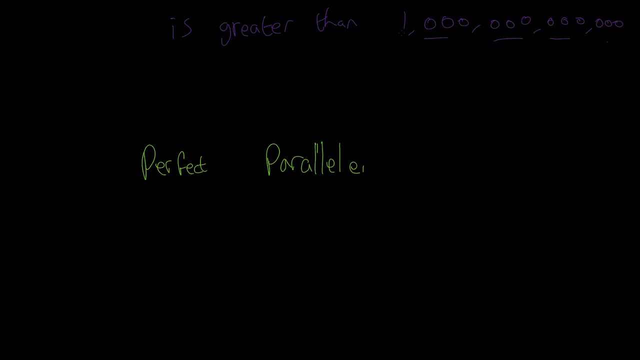 a perfect parallelly point. obviously, part of it is parallella, parallel parallella point. actually, I think I've got it, the parallella point, I believe that's the way it's pronounced, and this is you know what a parallel is, a parallelogram? I should say it's like this: